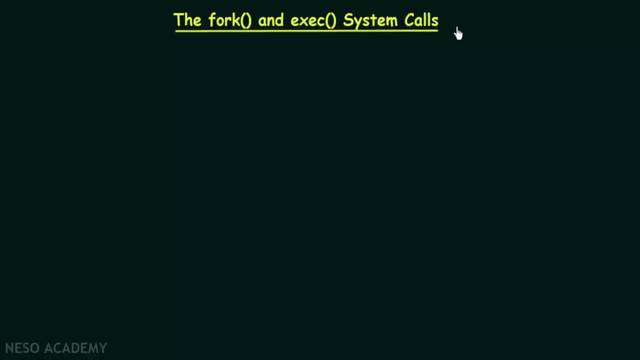 In the previous lecture, we have studied about multi-threading models and hyper-threading. Now the next topic that we need to discuss is about issues in threading. But before we go to the issues that we face in threading, there are two important things that we need to understand, which are the fork and EXCC system calls. 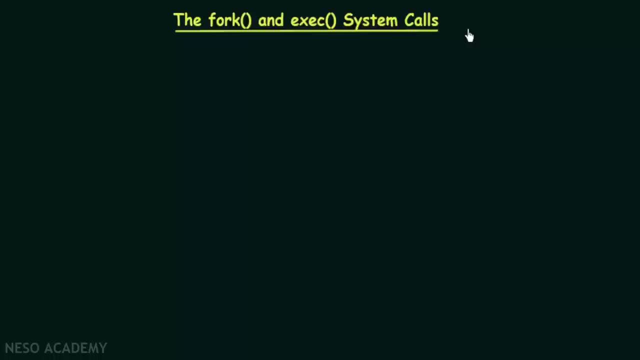 Now, after understanding the fork and EXCC system calls, we'll be in a position to understand the issues that we face in threading. Now I'll not be explaining the meaning of system calls again, because we have already done a lecture on system calls and if you have not watched it, 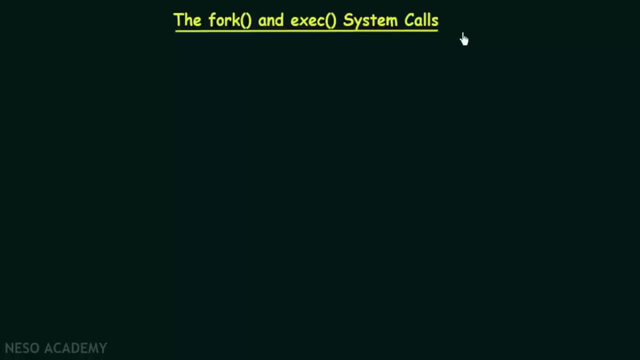 I request you to watch it so that you understand what system calls mean. Now, before we go into fork and EXCC system calls, let me also tell you that this fork and EXCC system calls are mainly specific to Linux-based systems and you may not be able to use it exactly like how I am going to show you in a Windows-based. 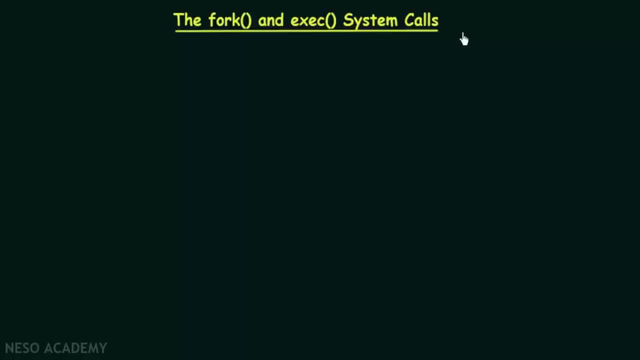 system. But here, since we are discussing about operating system as a whole, and since we are not focusing on a specific operating system, it is good to understand the issues that we face in threading. Also, if you are interested in learning in depth about operating systems, 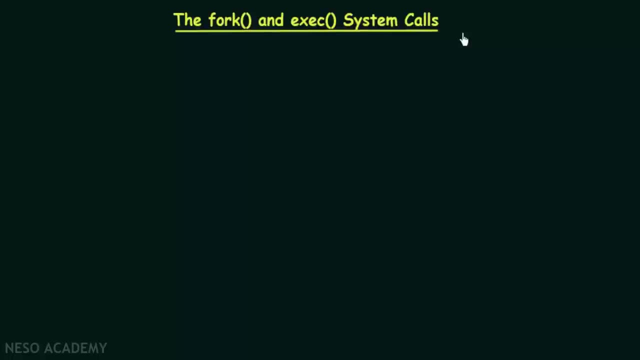 Linux would be a very good choice, because it is an open source system and hence you can see how it is written, and you can also modify it yourself and learn a lot from that. Alright, now let us see what are these fork and EXCC system calls and what do they do. 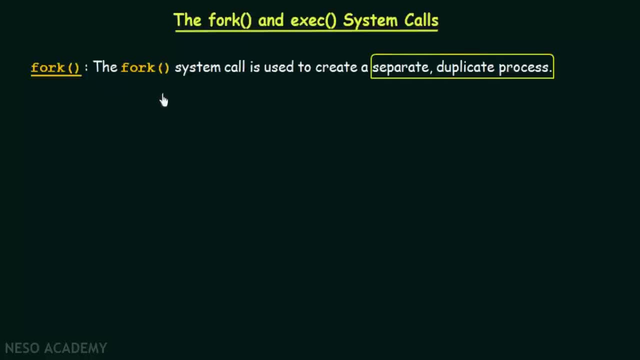 So, coming to the first one, which is the fork system call, the fork system call is used to create a separate duplicate process. So whenever a fork system call is used, a separate duplicate process of that same process from which it is called will be created. So suppose you are having a process running and 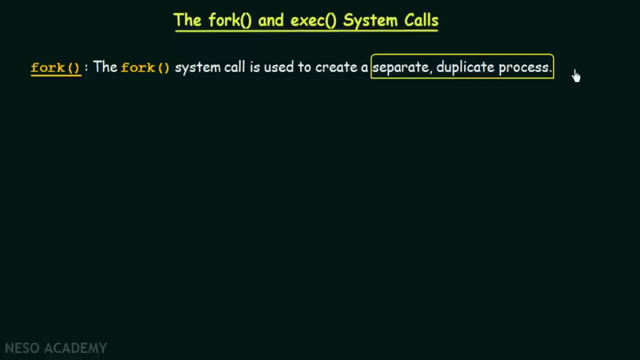 you want to create a duplicate or an exact replica of that process, then we use the fork system call. So if we are using a fork system call, a separate duplicate process, which will be exactly the same like the process from which it was called, will be created. 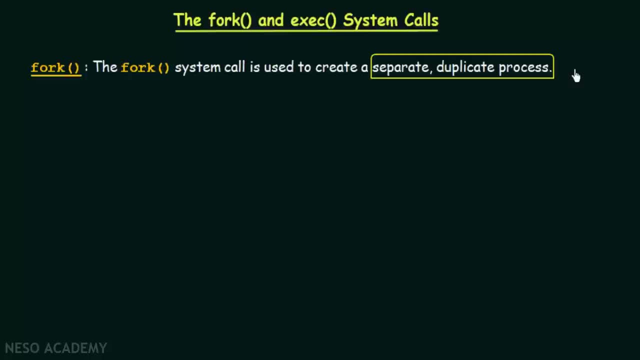 But the only difference is that the new process that is created will have a different process id. So the process from which where we call the fork is known as the parent process, and then the duplicate process that is created is known as the child process. So, as I said, this is an exact replica of the parent process, with the only 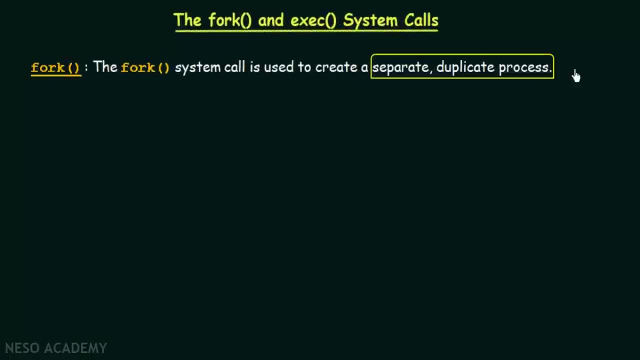 exception that it will have a different process id. Alright, now let us go to the next one, which is the EXCC system call. In this EXCC system call, what happens is, when an EXCC system call is invoked, the program specified in the parameter to the EXCC will replace the entire process, including all the 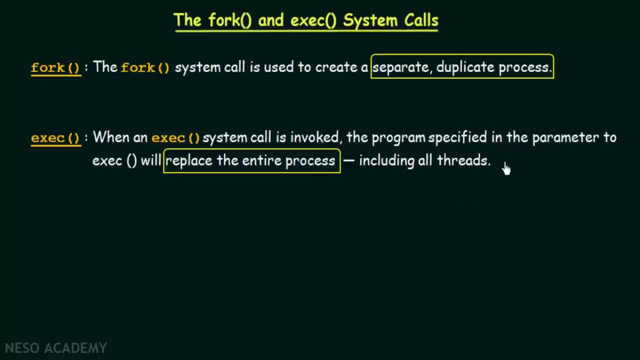 threads. So, unlike the fork system call, when you call an EXCC system call or when an EXCC system call is invoked, then we have to pass into this EXCC system call a parameter which will be another program. So when we pass a program into this EXCC as a parameter, then that program will replace the 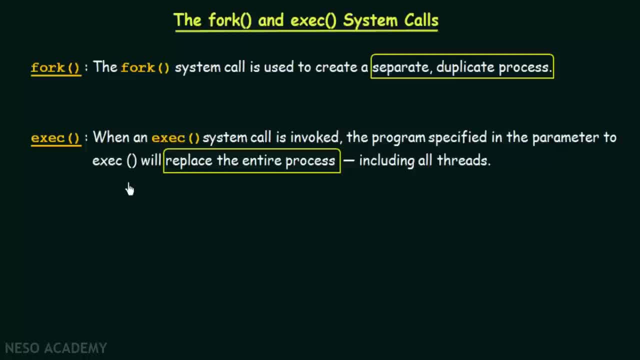 entire process from which this EXCC was called. We can understand in simple terms that EXCC system call is used to replace a process with another process, and then they will have the same process id, because here we are not creating a new process, but we are replacing an existing one, So the 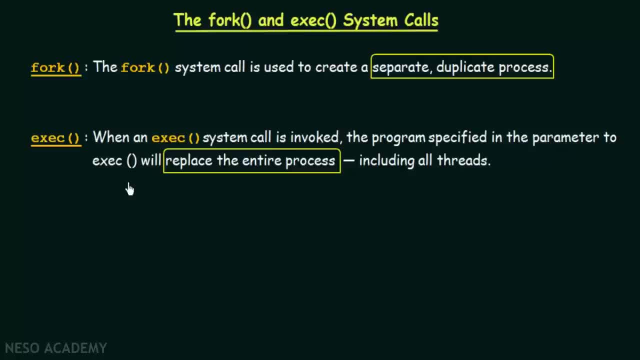 process id will remain the same, but the contents will be different. So that is what this EXCC system call is used for. Now we don't want to simply learn this definition, But let us try to see and understand how this fork and EXCC system call actually work. 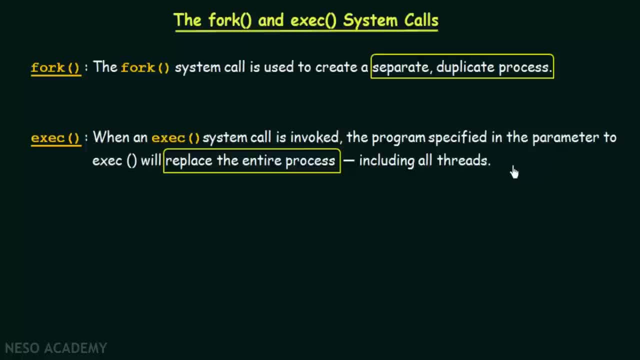 So we will be writing programs for this in C language and then we will run it and we will analyze the output and we will see how this fork and EXCC system calls work. As I told you in the beginning, these are specific to Linux based systems, So I will not be able to show you this. 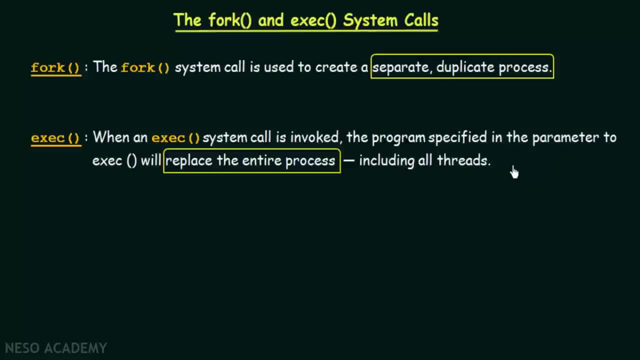 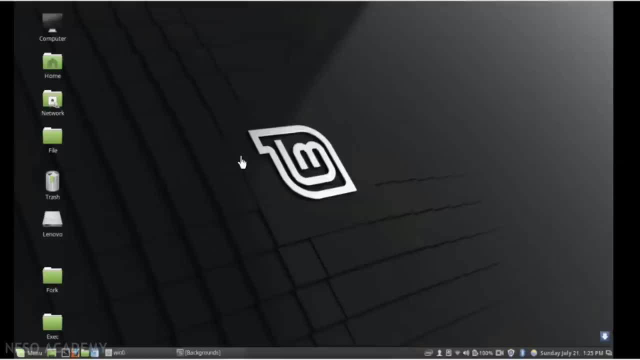 in Windows. So let me just switch over to my Linux system and there we will be writing the program and we will see how these two system calls work. So here I am on my Linux based system and I'm using Linux Mint, and here I have created two folders on my desktop called 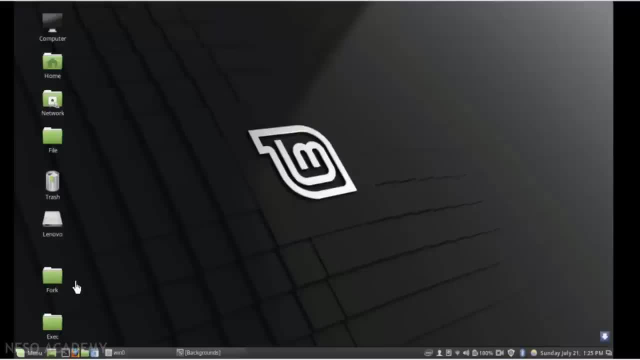 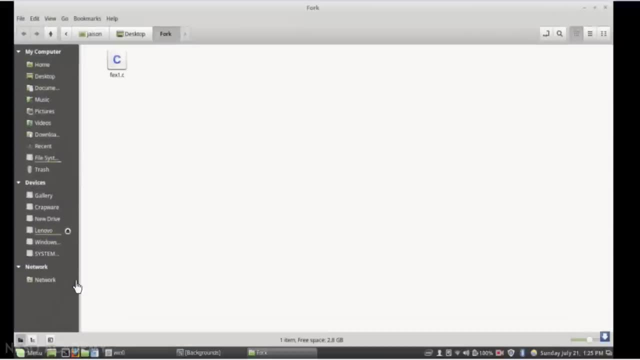 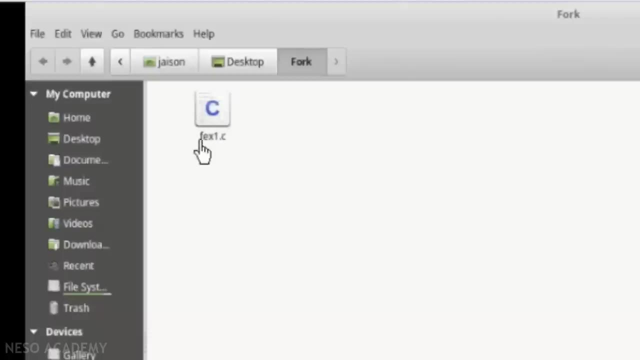 fork and EXCC, and inside these folders I have written the programs where we will be able to understand how fork and EXCC system calls work. So, coming to the first folder, here I have a file called fex1.c. This is a file in which I have written a program in C language. So let us open. 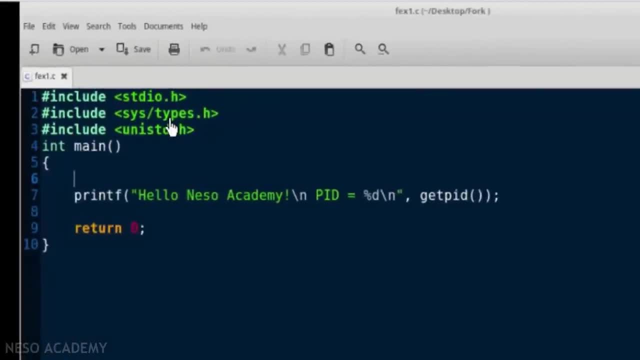 that up, All right. So here this is a simple program where we have declared a main function and then we are just printing one line over here. So the line here says: hello, nesso academy. and then it says pid equal to- and here I've used a function to get the pid, which stands for the process id. So what? 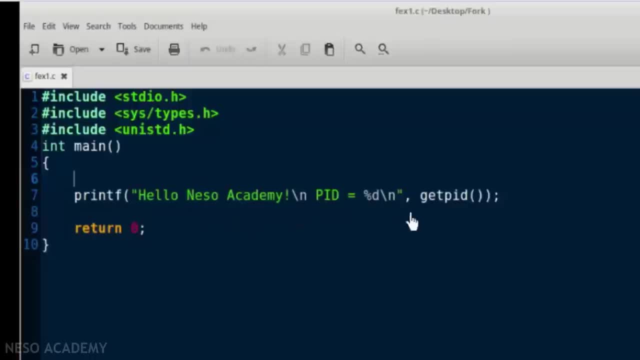 this program will do. it will just print hello nesso academy and it will print the process id of this particular process that will be running. So now, in order to run this program, let me go to the folder where this file was created, which is this fork folder. So let us open that up. So now here. 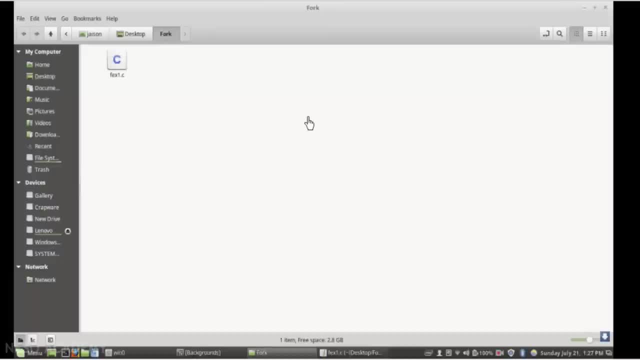 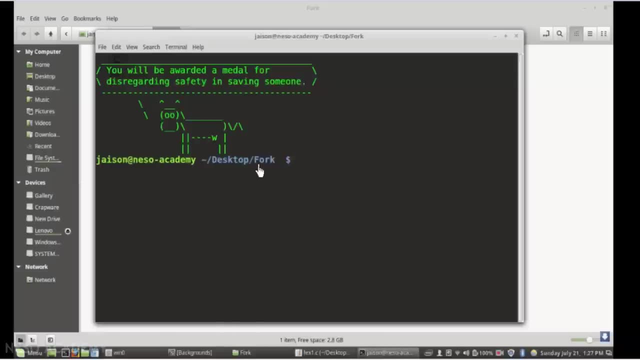 we need to open the terminal of our Linux For that. we just right click and click open in terminal and then the terminal will open for that particular folder which is in desktop, and the folder is named fork. Now, in order to run this, we type gcc space, the name of the file, So gcc is. 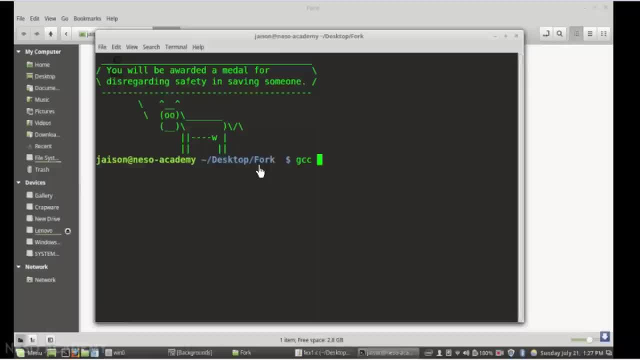 the compiler that is used in Linux in order to compile C programs. So we type gcc, followed by the name of the file that we created, which is fex1.c, and then you press enter. Now, when you press enter, this file is compiled and the output, or the executable file, would be: 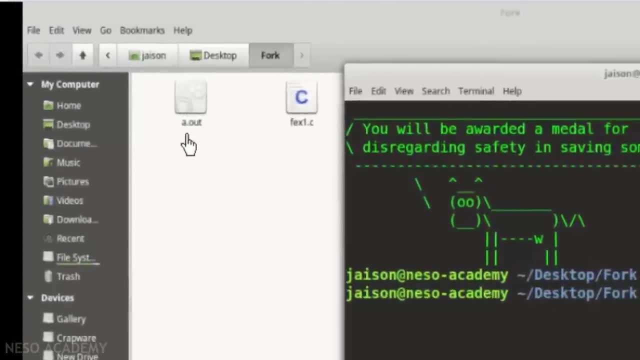 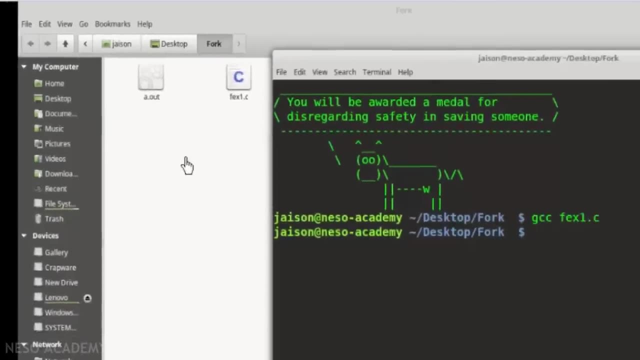 generated. Now, if you look here, you see that there is a file called aout. So in the beginning we only had fex1.c. Now, when we compiled it here, this aout file is created, which is the executable. we need to run this output file in order to get the output. So let us come back to the terminal. 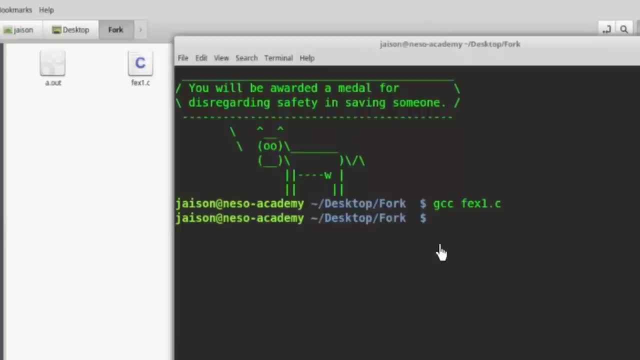 and do that. So in order to run it, what we have to do is we have to type dot: slash a dot out. So that is the command that we use, and when we run it, here we see the output: hello nesocademy. and. 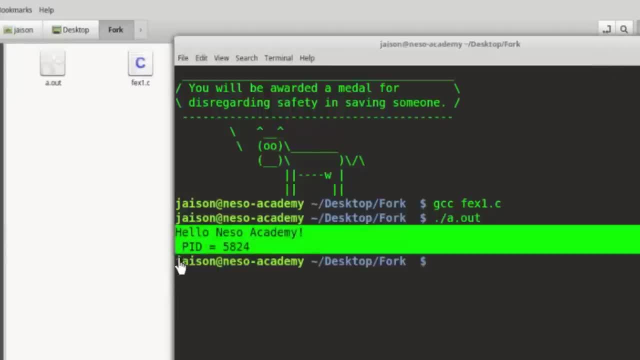 the process id is printed. So that is the output of our program. So that is all we did. We just printed hello nesocademy and the process id is printed, which is 5824.. Now what we will do is: 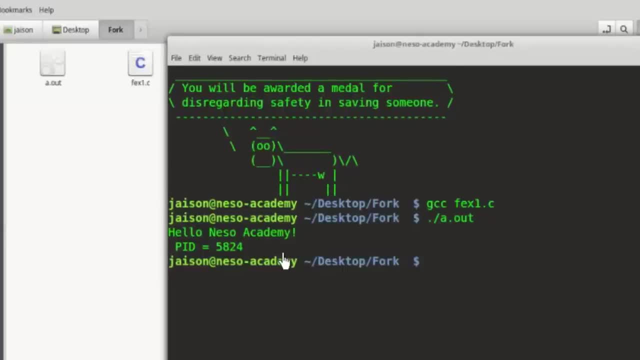 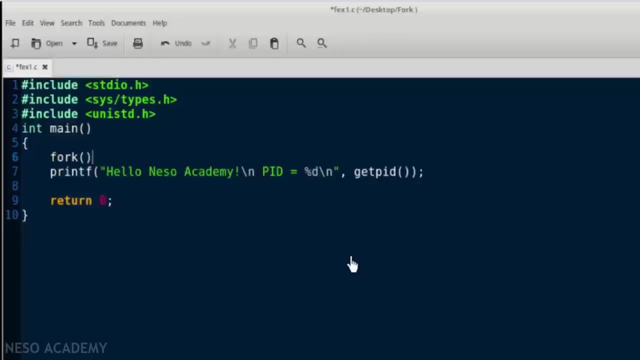 we will go back to the file and let us edit that program and put the fork system call into it and see how it works. Now we come back here and I will type a fork system call here, all right, and then let us save this program. Now, after saving it, we have to go back to the terminal and we have to 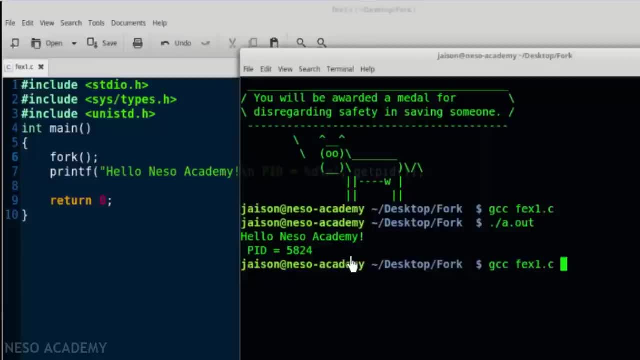 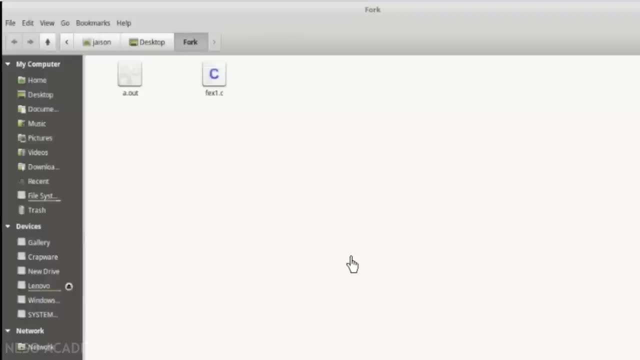 run this program. So we come back to the terminal and in order to run the program, we type the same command- gcc- file name- and we press enter, and then the output file would have been created. Now, if you look at this, in the folder there is a a dot out file was already there in the beginning. 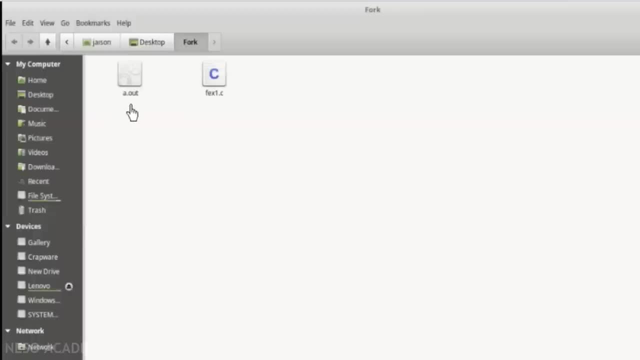 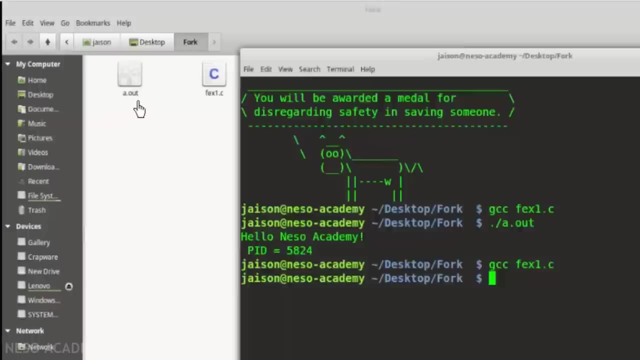 Now this a dot out file which is here now. this is the new a dot out that was created and replaced. Now we are going to run this a dot out in our terminal. So we come back to the terminal and type the same thing: dot slash a dot out, and here you see the output. it is printed: hello. 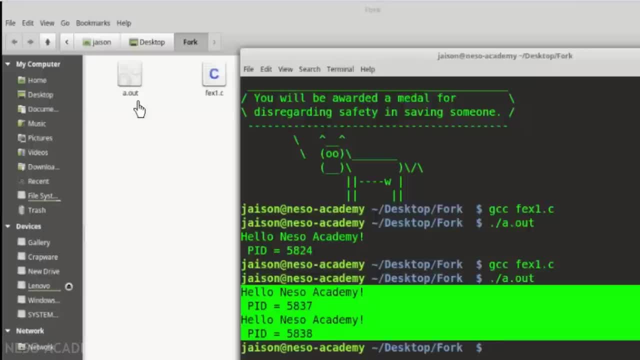 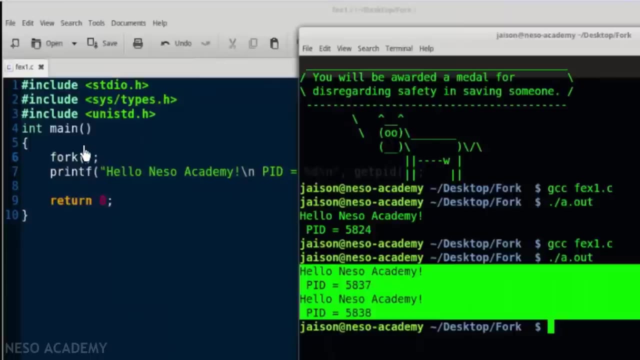 nesocademy with pid 5837. and again it is printed hello nesocademy with pid 5837.. 5838.. Now you see that the program was executed two times. and why is that? That is because of the fork system call. So if you look here, we type fork over here, and when we type this fork. 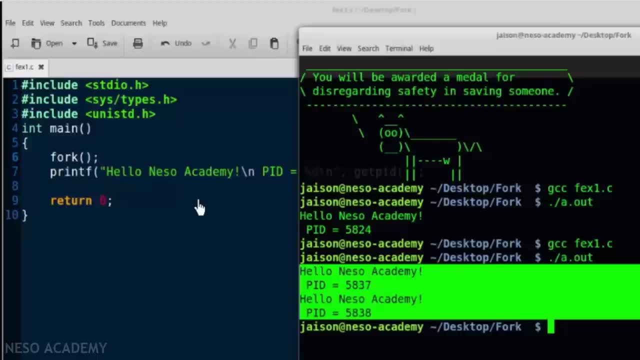 what happened was this program created its own child process. That means this process was executed two times, Once by the parent and another time by the child. So when this fork was used, Hello NSW Academy, with the first PID, which was 5837, is printed, and then the child process was. 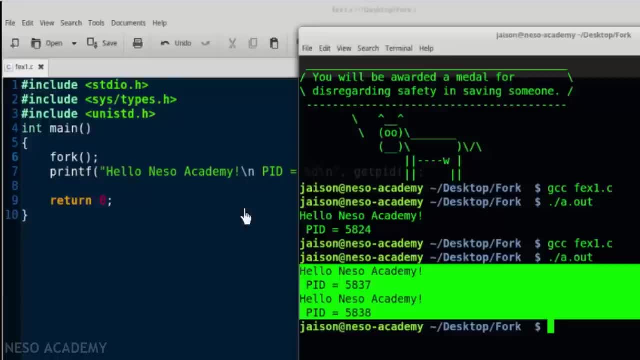 created because of this fork and that also got executed printing the same thing Hello NSW Academy with a different process ID, which is 5838.. So you see that the process IDs are different. So that is what I told you in the beginning: that when the fork system call is invoked, it will create a. 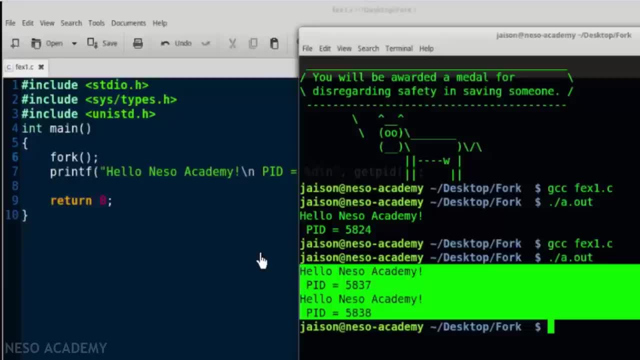 separate process with a different process ID, but the contents will be exactly the same. So that is why the same is printed, but just in order to show you the process ID, I have put this PID to make sure that they are different. Now let us do some modifications and try to find out if I come back. 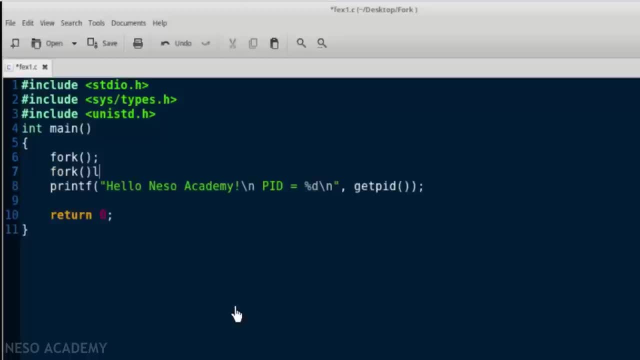 to this program and insert a few more forks. let us try to see what would be the output. So here I am coming and I am typing two more forks. So here now we have a total of three fork system calls and I have saved the program. Now, if I have this three fork system calls, what will be the 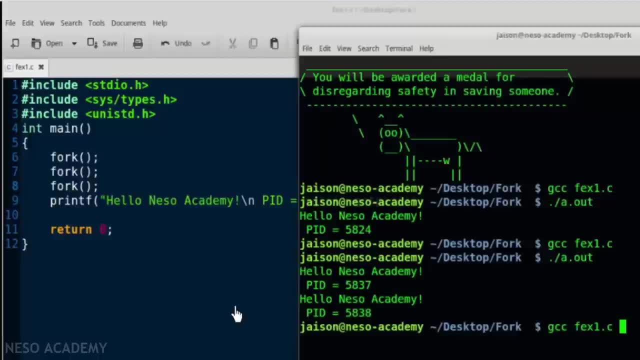 output of my program. Let us try to find that out. So we come back to the terminal and we compile the program gccfex1.c. Now, before I run this, take a moment to pause this video and think for yourself how many. 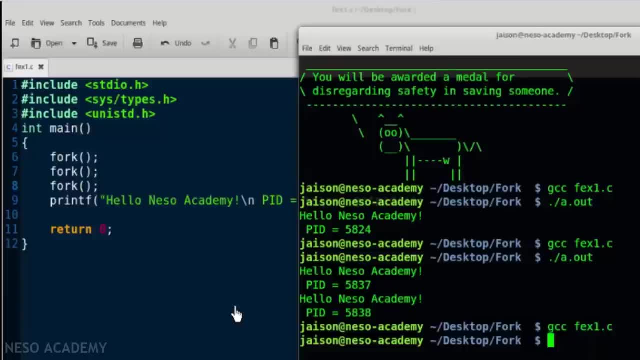 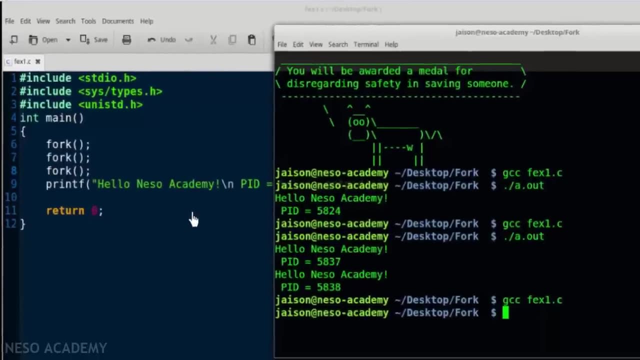 times will the print statement be executed when I have given this fork three times, and then we will see if you got it right. Alright, now let us try to run the program again. So we type //aout, and let us see how many times is it printed. 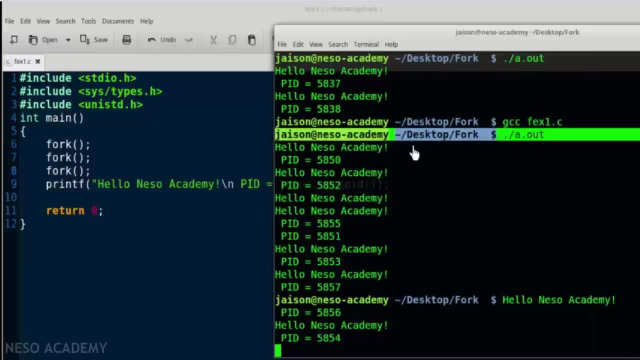 Okay, so here we have our program. So let us try to run the program again. So we type //aout and let us see how many times is it printed. Okay, so here we have our output From here. if we check, this is where we ran it and it is printed 1,, 2,, 3,, 4,, 5,, 6,, 7,, 8 times. 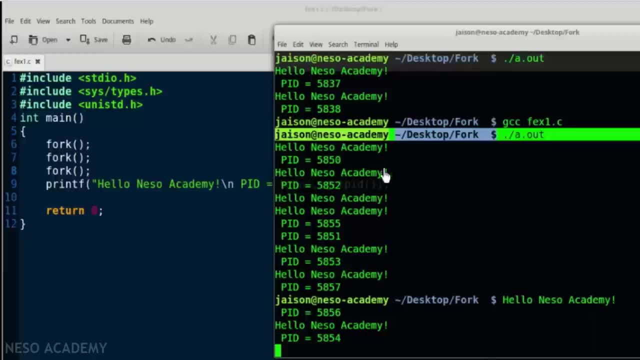 So when we put three fork system calls, it was executed 8 times and in all of the 8 times it is having a different process ID. Here it is 5850,, here it is 5852,, here it is 55,, 51,, 53,, 57,, 5654. 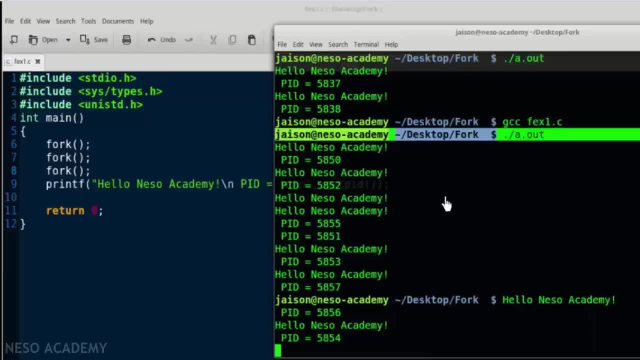 So it is having a different process ID at each of the times. Now can we understand why is it printed 8 times? So, first of all, what happened is that we have the first parent process, which is P1.. So let me call it P1, which is the first parent process that is there. So it will print. Hello. 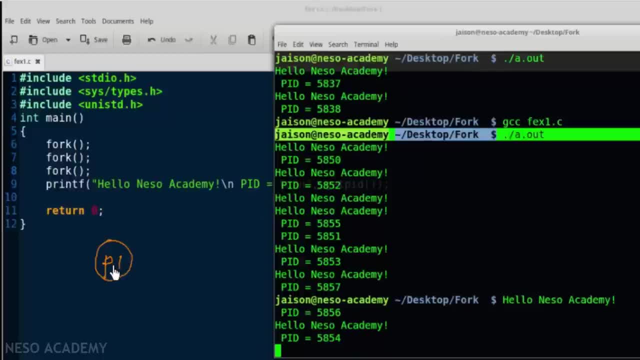 NSO Academy with its PID just one time. So that is what it will do. So that is the first process that is there. Now, when this first fork was executed, what will happen is this process: P1 will create its own child process. 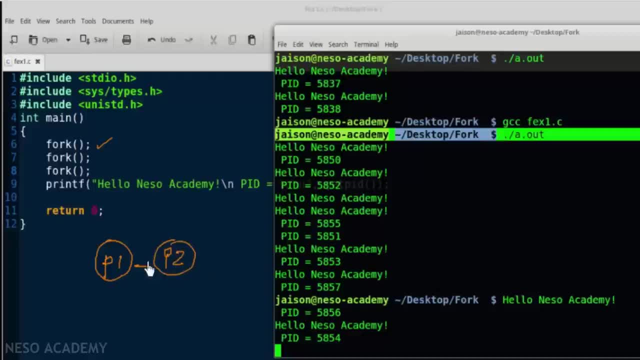 Let me call it P2.. So P2 got created and now there are two processes. Now what happens is, when the second fork system call is executed, then we see that there are two processes. now in our system There will be child process created for each of these two processes. 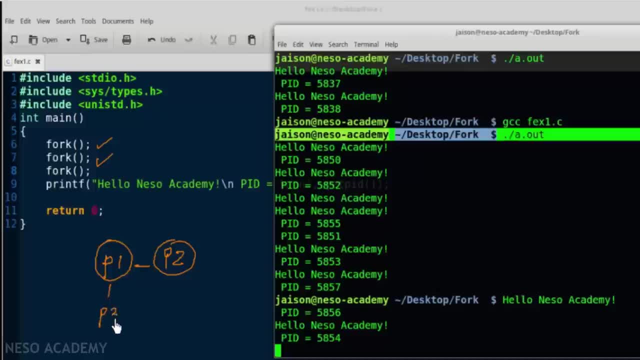 So for P1, it will create another child process- Let's call it P3- and for P2, it will create another child process, P4.. So we have a total of four processes. Now, when the last system, call or fork, is executed, what will happen is here we see. 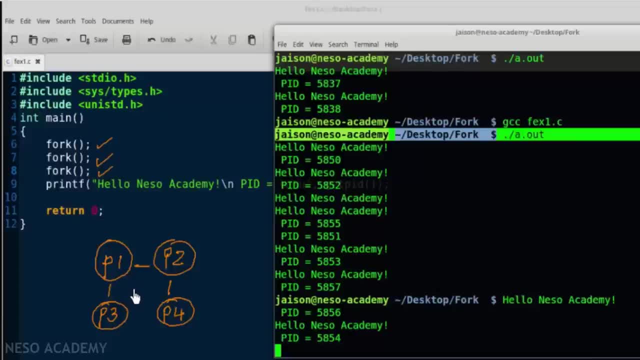 there are four processes now, and for each of these four processes there will be one child each created. So let's say, for this P1, it will have another child process called P5, and for P2, it will have another child process. 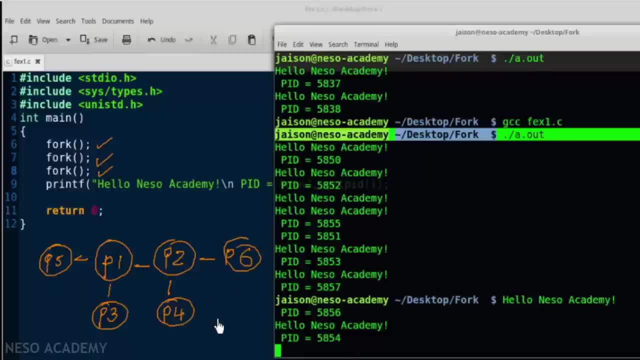 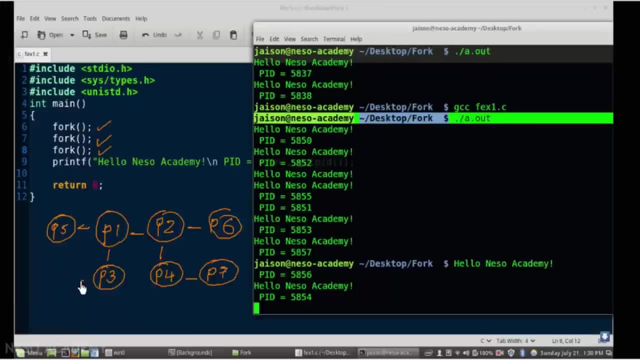 Let's call it P6. and then for this P4, it will have another child process. Let us call it P6.. Let's call it P7, and for this P3, over here also, it will create one child process. Let's call it P8. 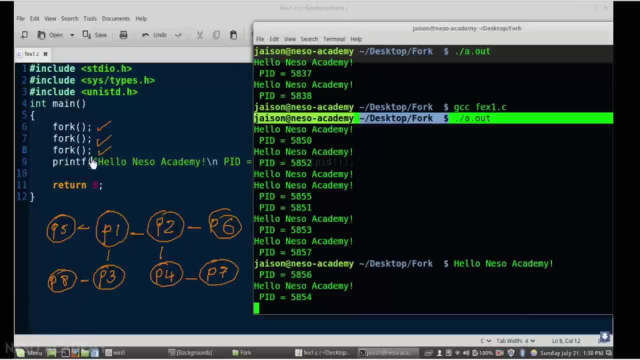 So these are the number of processes that will be created- Now there are no more fork system calls- and how many are created. Eight of them were created and that is why Hello NSW Academy was printed eight times in this output. So here we see, for each of the times it is having a different process ID. 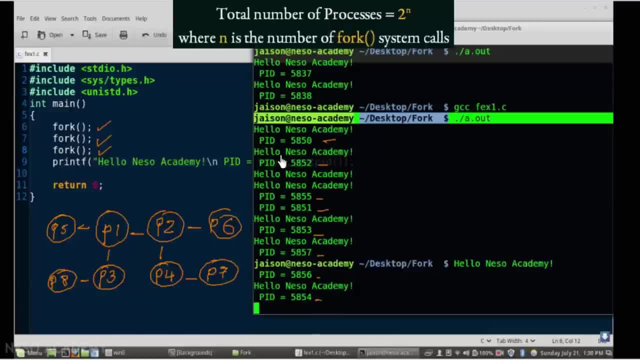 So the thing is they are all new processes but the contents are the same with different process ID. So that is what happened when we use the fork system call. So I hope with that it is clear to you how the fork system call works. 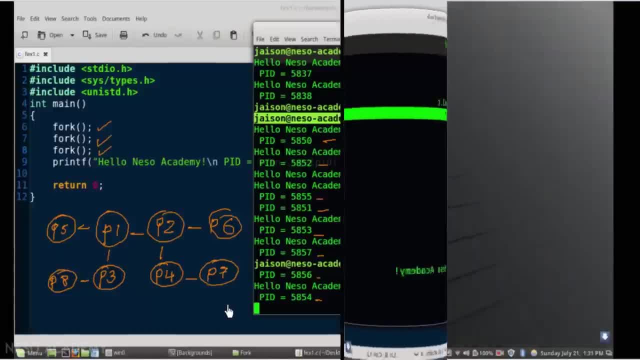 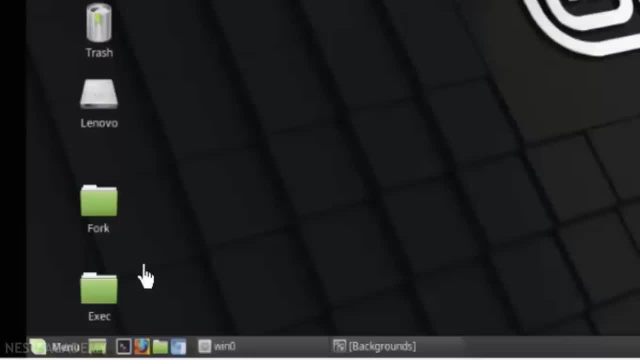 Now let us go to the next one, which is the EXCC system call. Now I will come back to the next folder that I have created, which is the EXCC folder, where I have written two programs in order to make us understand how the EXCC system calls work. 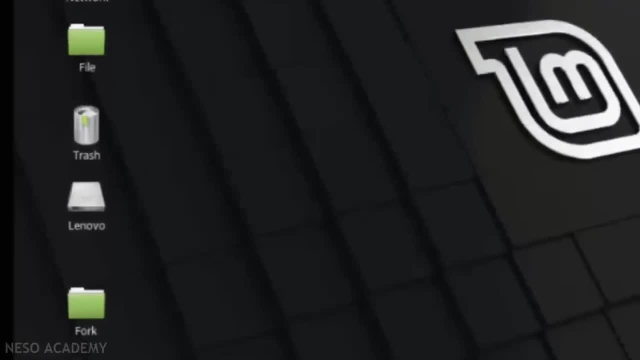 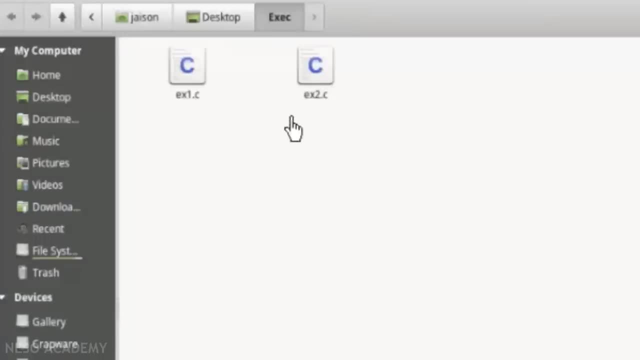 So let's go into that and see what does. So as we enter this folder, we see that I have created two C programs: ex1.c and ex2.c. So these are two C programs. So let us see what is inside these programs. 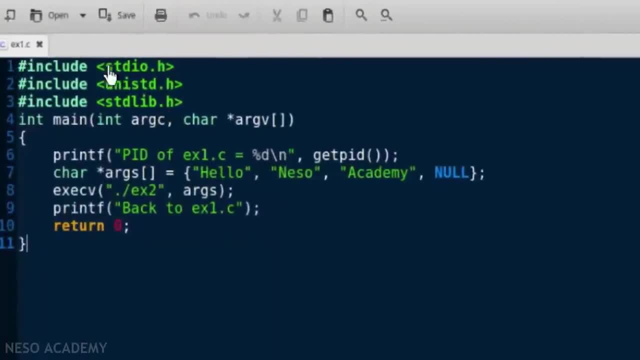 So inside the first file, which is ex1.c, here I have written a small program where there is a main function with some arguments, and then here inside main I have printed the PID of ex1.c. Okay, That means the process ID of this program will be printed. 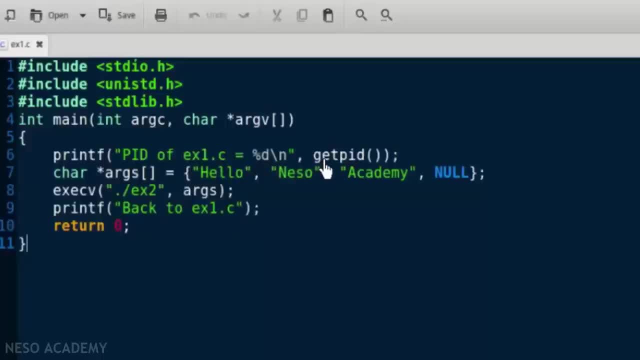 So here PID of ex1.c is equal to. and I am using the function getPID to get the process ID from the system, And here I have declared a character array where I have put in the words hello, nesso academy, and the last one is null. 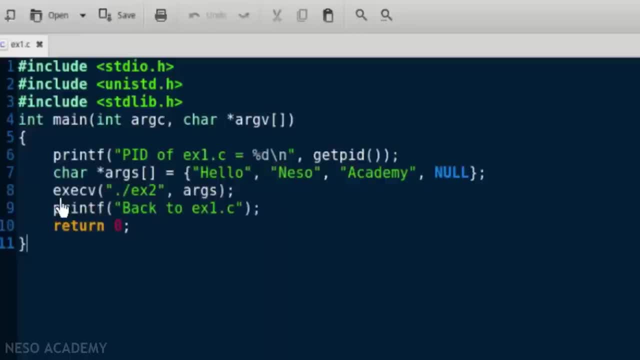 And after that we are using the EXEC system call. So here it is written: EXECV. So there are different type of EXEC system calls within the family of EXEC. So this is one among them, and I will not be explaining each of them separately, but 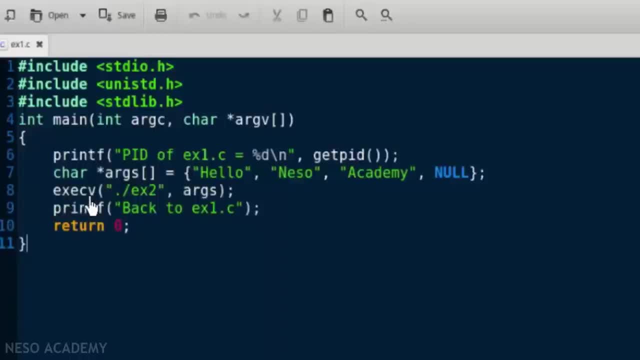 just know that this is an EXEC system call. And here what we are doing is we are passing as an argument the output of ex2, program that we have written. So ex2 was the next program that I have written, So this is ex2.. 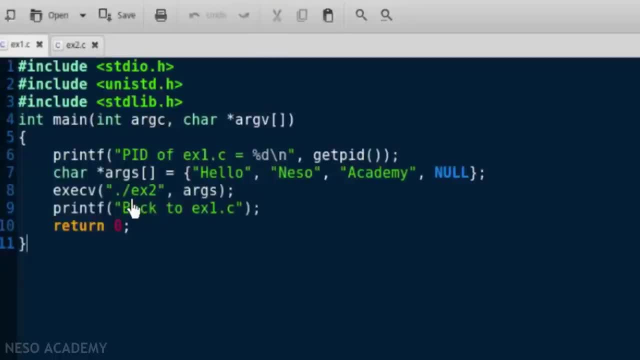 So I will be showing it to you later. Here I have written the output of ex2 and that is passed as an argument to the EXEC system call And then it is written here: another statement: printf back to ex1.c and return 0.. 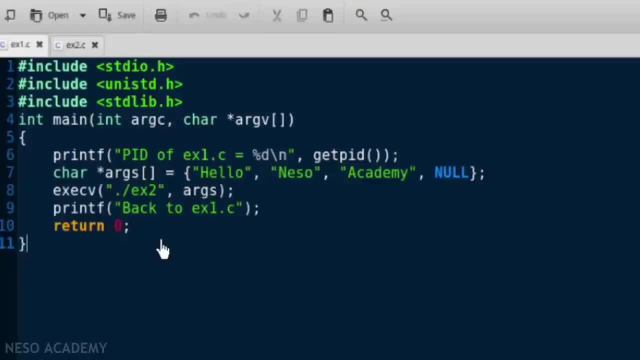 Now let's go and look at the next file, which is ex2.c, and see what I have written there. So, coming to this ex2.c, here again, similarly, we have a main function with some arguments, and here we have just written two printf statements. 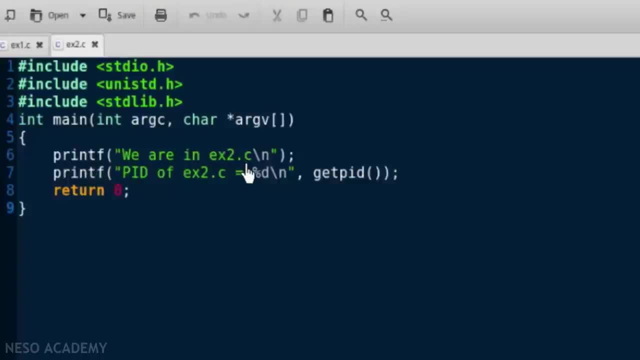 The first printf we are just displaying. we are in ex2.c. We are writing this so that when we enter into this ex2, this will be printed and we know that we are in ex2.c. So we are going to print the process id of ex2.c and then the pid of ex2.c will be printed. 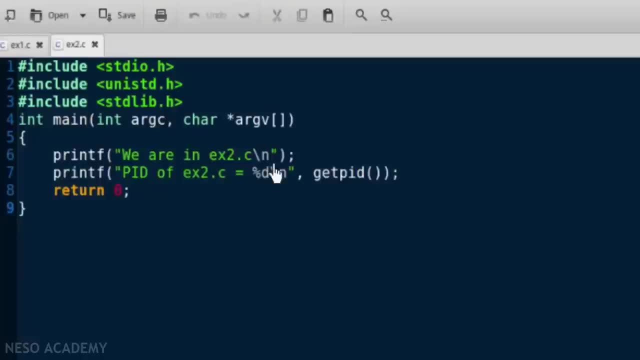 That means the process id of this particular program or process will be printed here using the getpid function. Now let us try to compile these two programs and run just one of them and see what happens. So, in order to compile these two programs, what we have to do is we come to the folder. 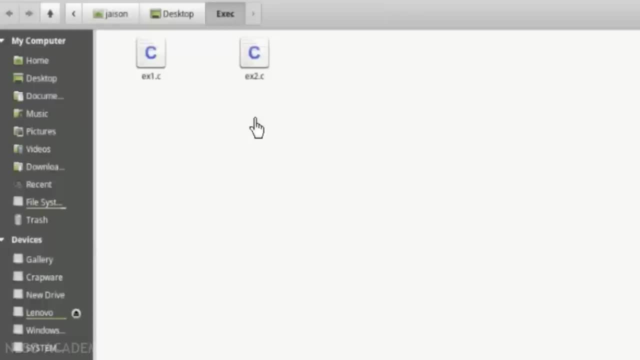 where they are present, and then we right click and open the terminal And then we have to type the same thing, that is gcc space- the. So we have to type the same thing. that is gcc space- the. So we have to type the same thing, that is gcc space- the. 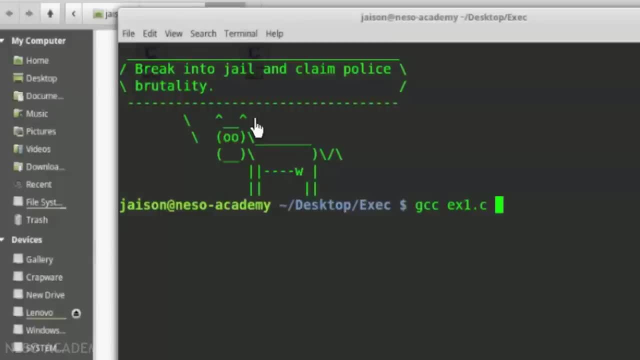 So we have to type the same thing. that is, gcc space. the. The first one that we are going to apply is ex1.c. One thing that you have to keep in mind here is that when I showed you the previous program of fork, we saw that when we compiled the programs in the GCC compiler of Linux, what it does- 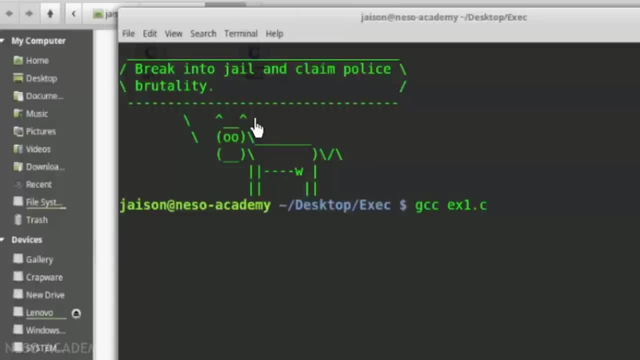 is, it will create a default output file with the name aout. So aout is the default name of the output file that is going to be created. but here, in this case, we are going to compile two programs, ex1.c and ex2.c, and since they are residing, 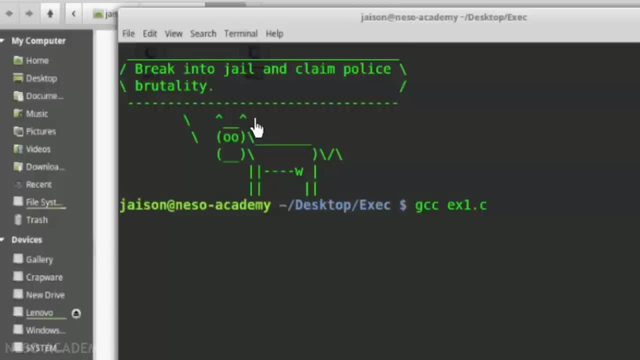 in the same folder. So here what will happen is that if I don't specify a different name for the output files of these two programs, when I compile this ex1.c, it will create a default aout file. After that, when I compile the next program, which is ex2.c, then the output file that 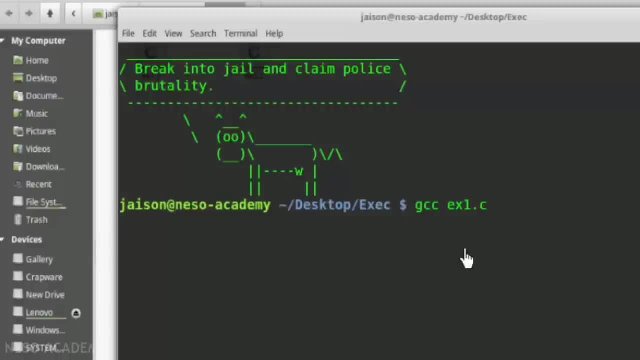 is generated for that is also named aout and that will replace the first aout which was created by this ex1.c. But we don't want that to happen, because we need these two programs. So in order to do that, we have to specify the name of the output file specifically. 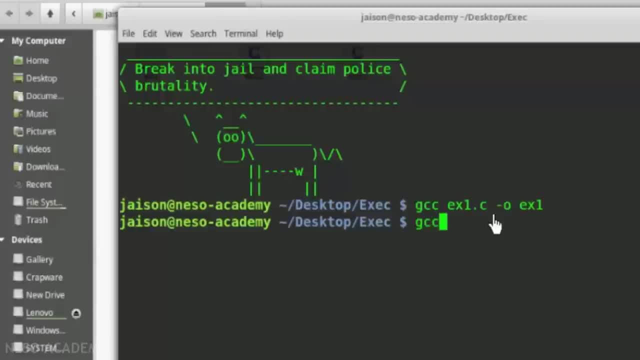 We have to type hyphen o and we have to just specify a name, like I have done here. This ex1 is the name of the output file that will be generated for ex1.c Now. similarly we can do for the next one. So ex2.c and hyphen o: ex2.. 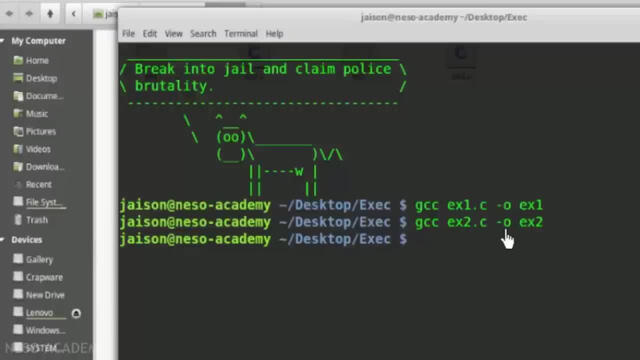 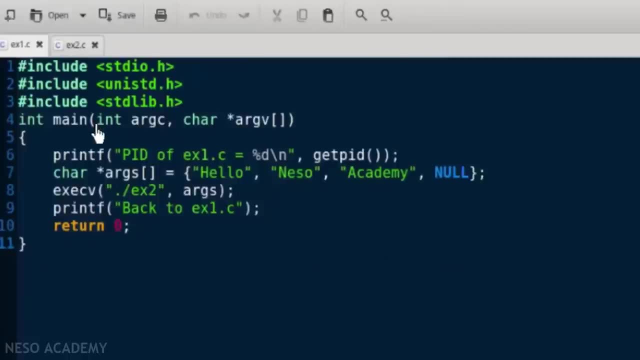 Here what happened. I compiled ex2.c and the output file. I have specified the name as ex2.. Now, before we compile the output file, we have to specify the name of the output file. So before we run this, let us come and take a look at this first file, ex1.c, again. 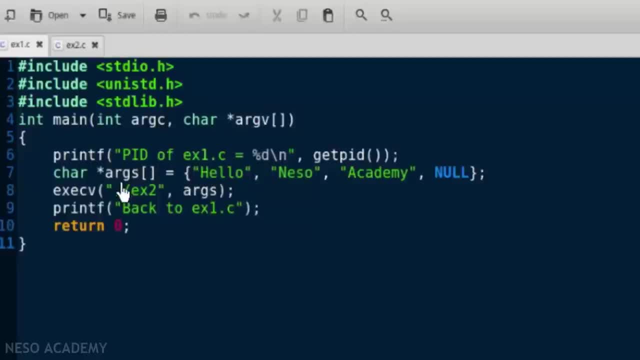 So here what should be printed: PID of ex1 should be printed. Then here we have declared HelloNASA Academy and here we are invoking the exec system call and as a parameter or argument we have passed the output file ex2.. That is the output file of the second C program that we have created, and then it prints back. 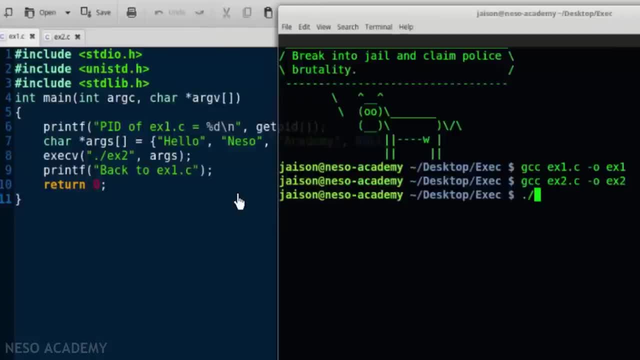 to ex1.c. Now let's see what will happen when we run it. So we type / And the name of the output file is ex1.. We are just going to run the first one Now see what is the output. So let me move it here and let us closely examine what happened when we executed ex1. 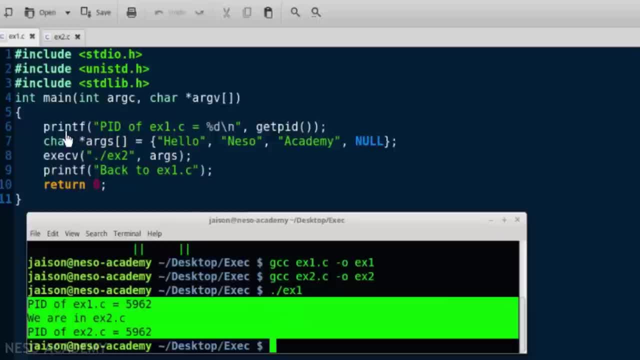 So ex1 is the output of this ex1.c. So here what happened. it came here and it printed the PID of ex1.c, which is equal to 5962.. So it printed this line over here. Then here we just declared this character array. 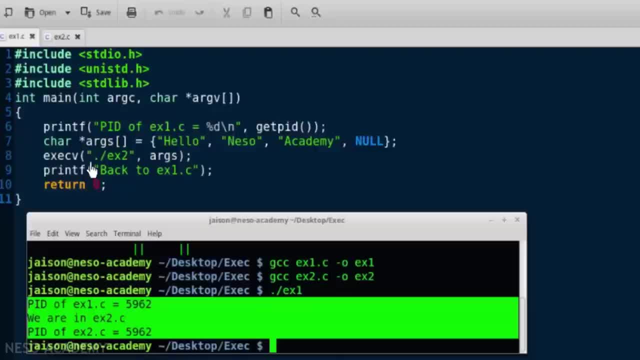 And then here We are, invoking the exec system call. And what did we pass as an argument ex2, which is the output of the second program, which is ex2.c. And then let's see what happened. Here it is written: we are in ex2.c now. 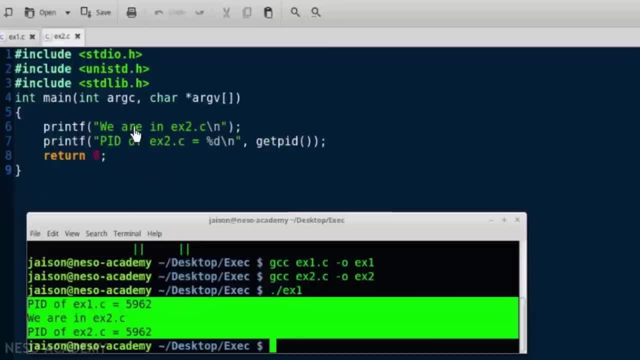 Now, why did that happen? Check this ex2.c Here. we are in ex2.c. it is written: we are in ex2.c. We are in ex2.c. So we see that from the first program when we invoke the exec system, call it jumped. 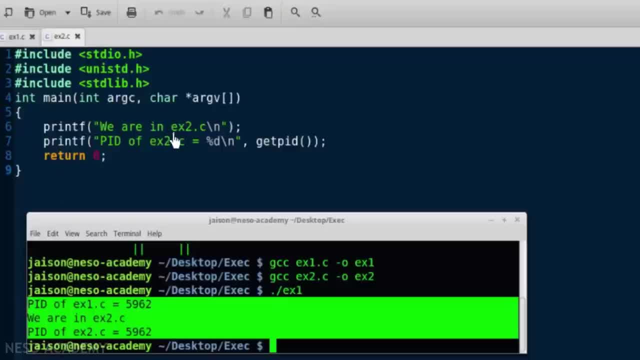 to this program, Right, And then it printed: we are in ex2.c and then the PID of ex2.c is printed. What is it? PID of ex2 is 5962. So basically, what happened is it did not jump. What exactly happened was that when we call the exec system, call the content of the first. 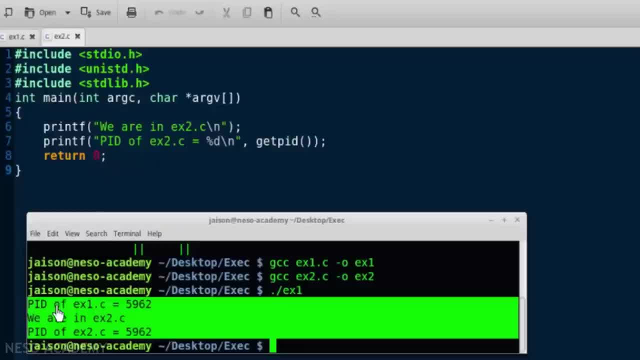 process was replaced by the second process. So that is why, after the first line, these things were printed, which is the content of this second program, ex2.c. And if you observe it, we see that the PID, or the process ID, remains the same. 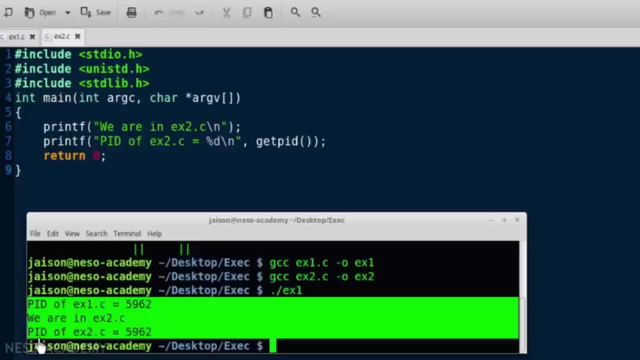 So when we were in the first program, the process ID was 5962.. And when we are in the second program, the process ID is still 5962.. So we see that the process IDs remains the same. exec system call will replace the contents. 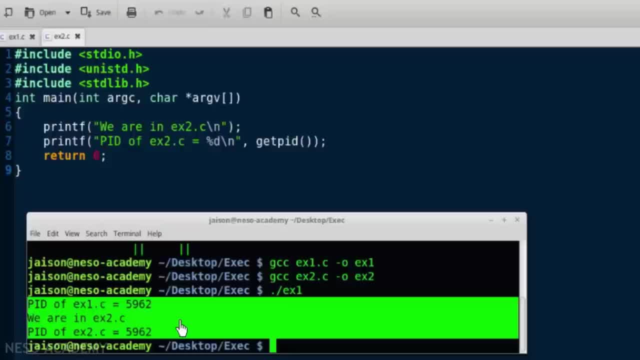 of one process with another process. So it is not creating a new one, but the first one is replaced by another one. That is why the process ID is the same, But the contents are now replaced. We only executed one of them, and from that we came to this. 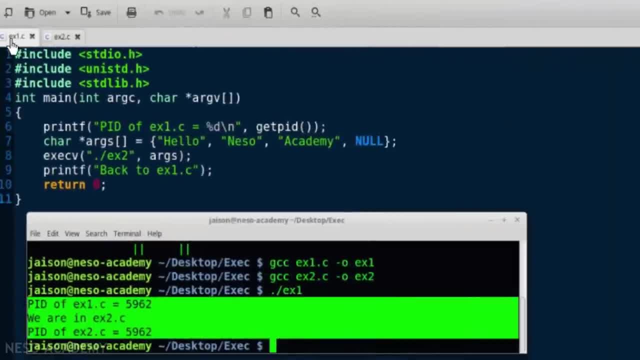 So that is how exec system call works. Now, if we come back and look at this first program, ex1.c, we see that there was one more line to be printed back to ex1.c which is not printed in our output. Why is that? 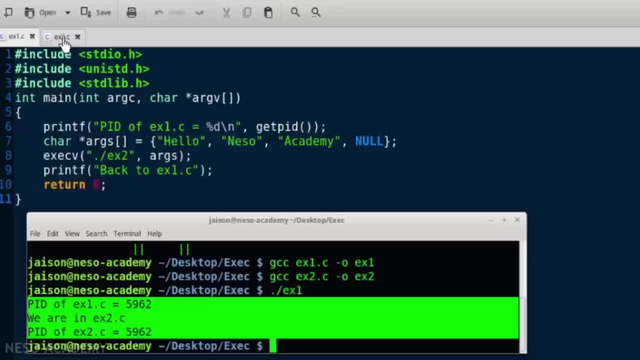 That is because when we entered this ex2.c in this second program we did not specify anything for it to go back to the first program. So it never had the control to come back to this first program again. So that is why this portion is not printed. 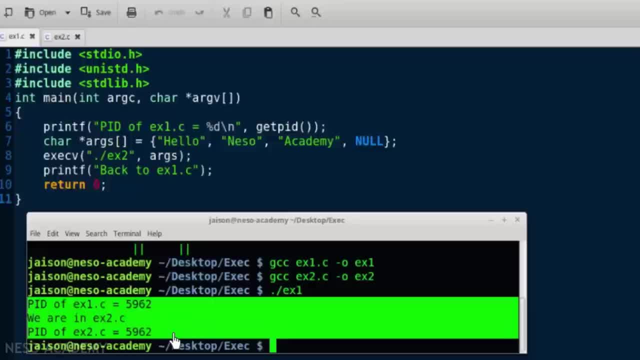 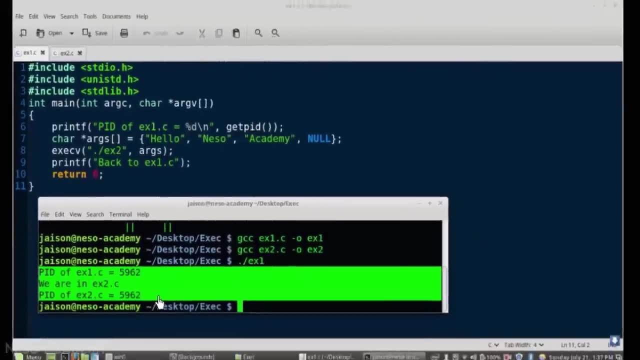 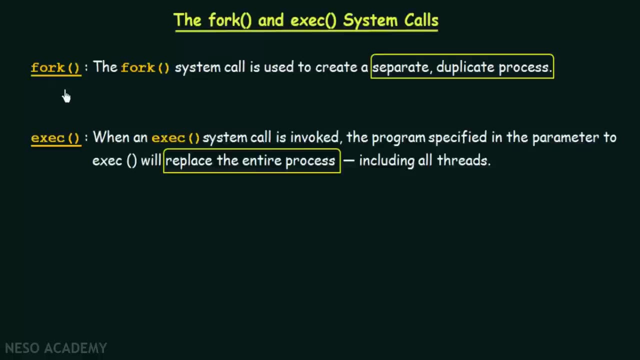 So that is how exec system call works. It replaced the contents of the process with another process, So the processes have the same process ID. That means it is the same process but the contents are replaced. So with that I hope it was clear to you about how fork and exec system call works.